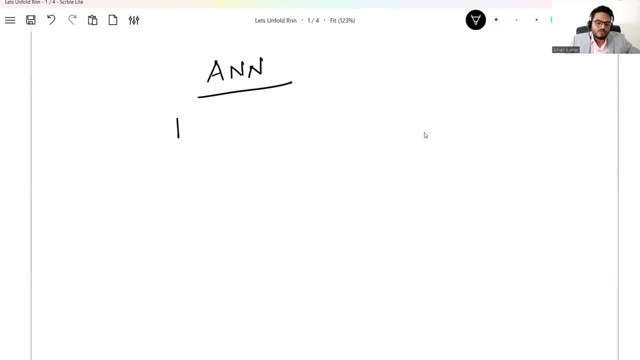 be familiar with the concepts of: what is the meaning of bias? What is the meaning of weights, OK, and because I'll be using these terms in the explanation- and what is the meaning of training of a neural network? What is the meaning of forward propagation? What is the meaning of? 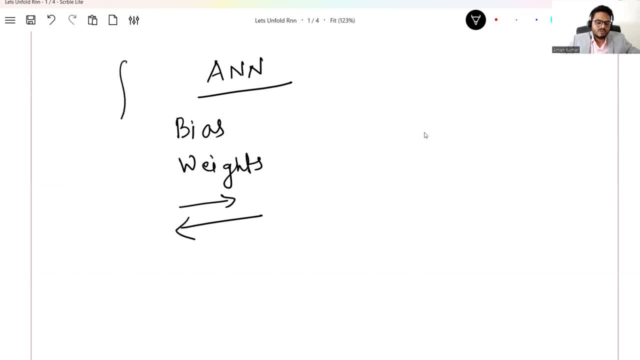 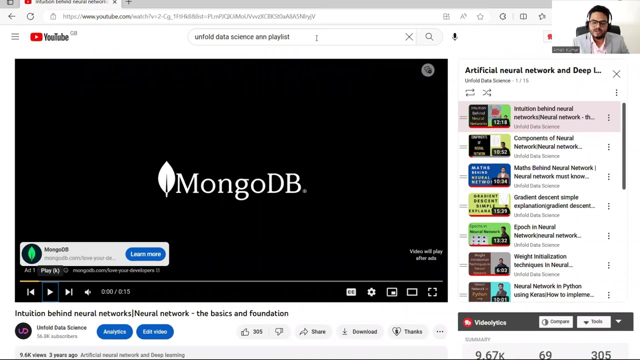 a backward propagation. If you have confusion on these basic topics of neural network, I will advise you to pause this video and go to unfold data science playlist on artificial neural network. So you have to go to YouTube and search for unfold data science ANN playlist and you will find. 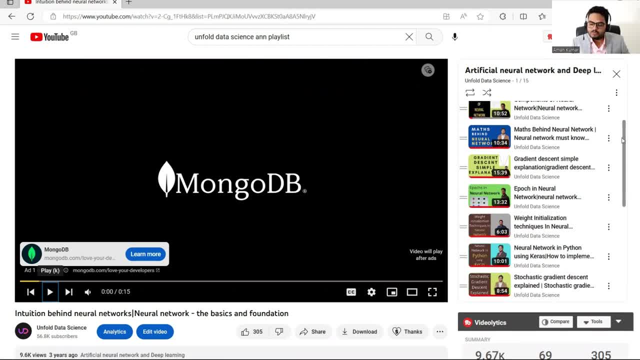 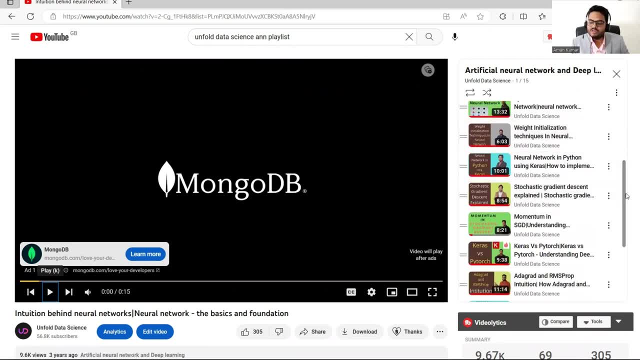 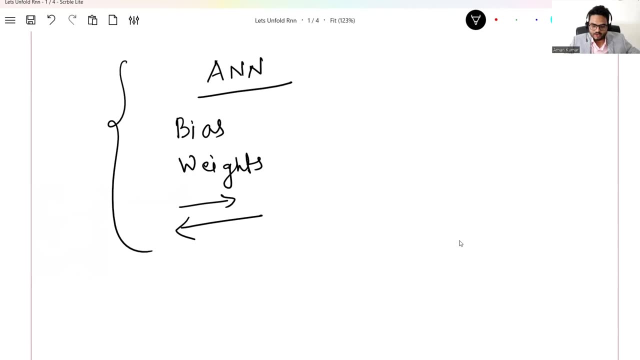 the videos. As I was telling you in last video as well, I am writing a sentence here, For example. I am same sentence here, the same sentence here, and the same sentence goes on right from scratch. components of neural network to maths behind neural network, to gradient descent, to epochs, to weight in initialization. 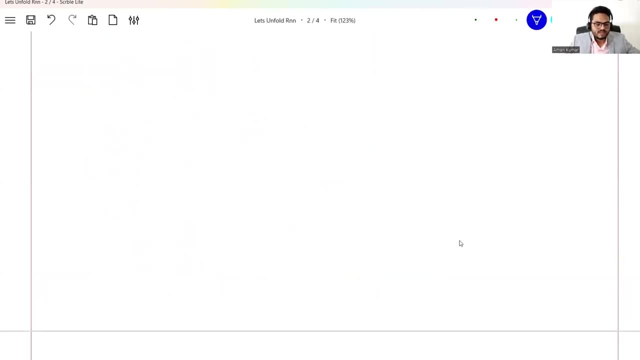 everything you will get here, OK, but if you are comfortable with those concepts, then let's move. I'm same sentence I will write here. so I was born. I was born in Germany. Germany, hence I can speak, and at the moment I say hence I can speak and fill in the blanks if I give. 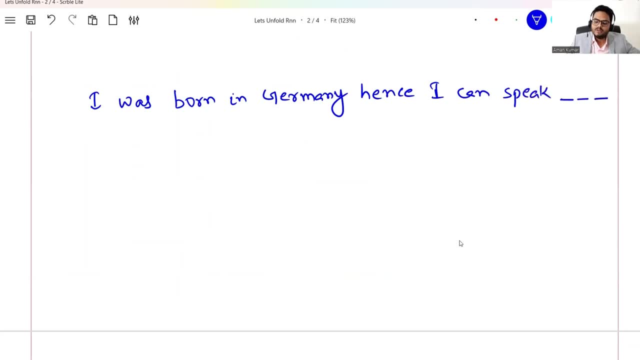 you write, you will be very easily say that you know here it should be German. okay, you should fill this blank with German. how are you able to say that? because you are able to relate from the previous information. okay, so if I give you just one information for 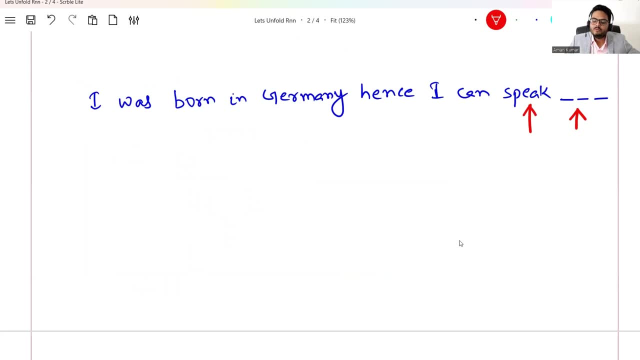 example, if I give you just speak word, maybe you will not be able to fill this, but since I am giving you everything, right from starting to end, you are able to derive that meaning and you are able to fill this. that is how human mind works, but unfortunately, computers. 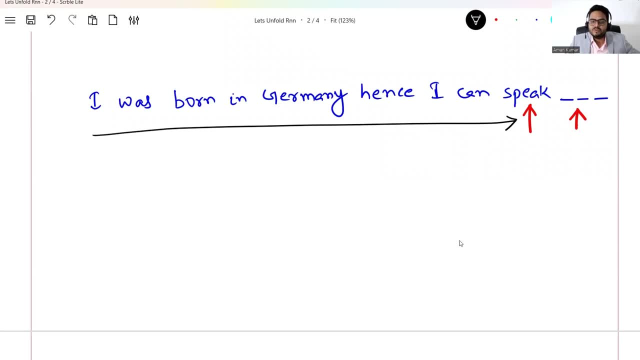 do not work like this until or unless a specific, you know a specialized network, it built in such a way. so that is where RNN comes into picture. so what RNN does is- if anybody asks you how RNN is different from basic neural networks, so there is only one word that differentiates: 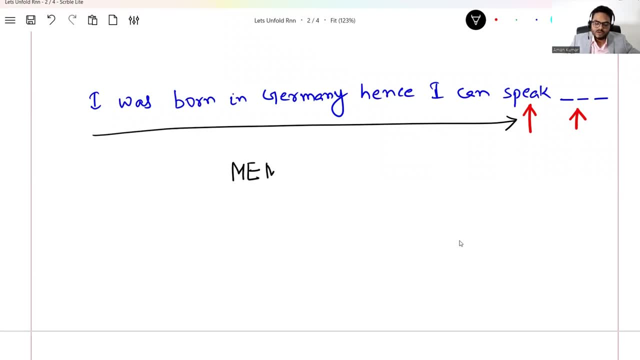 RNN from the normal neural network, and that is memory. okay, this is the one word that differentiates RNN from normal artificial neural network. memory means RNN has a capability of memorizing things. memorizing things means what memorizing things means, if I am at this word okay. so, for example, 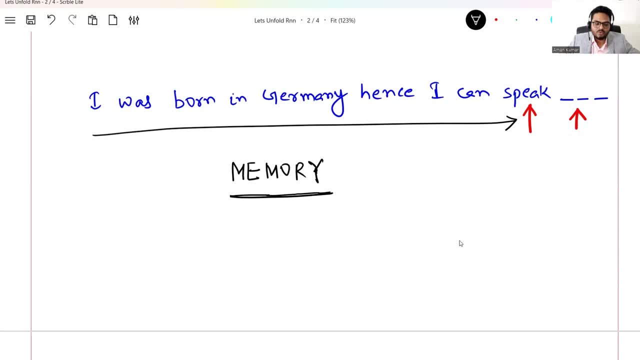 I will write here, for simplicity. I will write here word one, word two, word three, and you can go up to here, let's say, word n, okay, so when I am at word n plus one, then I remember. I remember what happened at word two and what happened at word three and what happened at 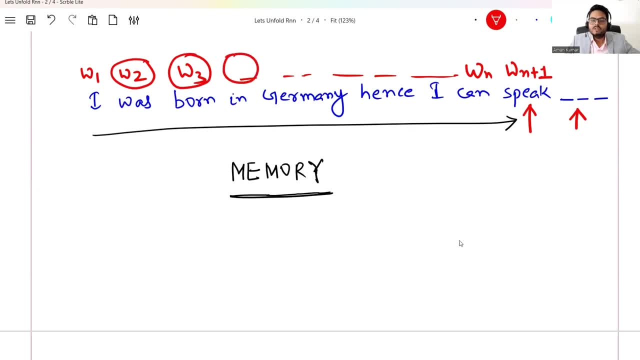 word four that that is the only thing that makes RNN different from normal basic artificial neural network. okay, and as I give you this example, if you do not remember the context, then you may not be able to derive this word with a meaningful derivation. so that is where 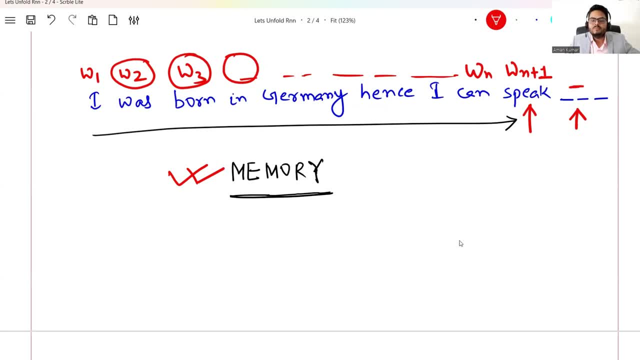 RNN was very, very useful because, as the as we go on to analyzing the complex neural networks, natural languages, the context becomes really, really important. okay, and in the world of RNN, what is the meaning of recurrent? so we will try to understand this, but first let me give you a 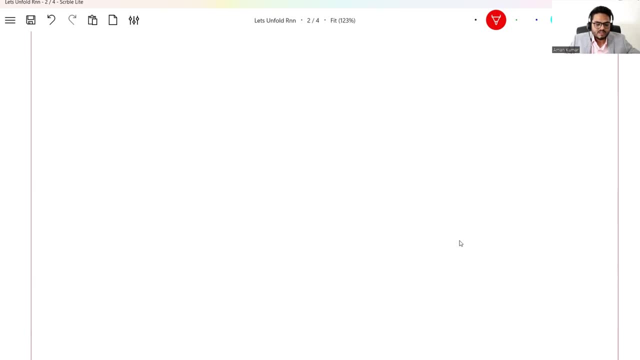 little background of, so that you don't confuse. let's say, I have in my, in my corpus, I have two documents, okay. my document one is: I'll give you a simple example here: my document one is: sky is blue, okay. and my document two is, let's say, sky is black, okay. so how many words we are having, how many? 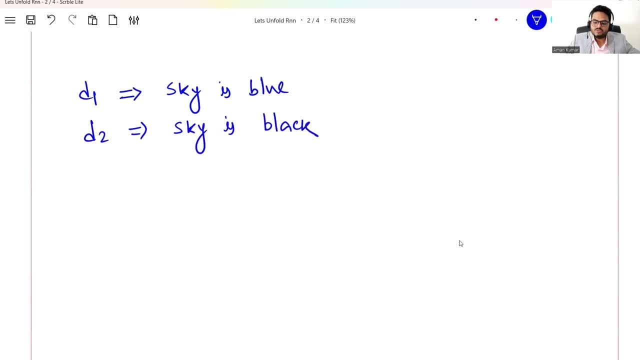 sentences or documents. we are having two. how many words we are having here? just let's count the number of words. first word, unique words, I'm counting, okay. second word, third word and fourth word. so in my corpus, just four unique words and how many documents? two different documents. 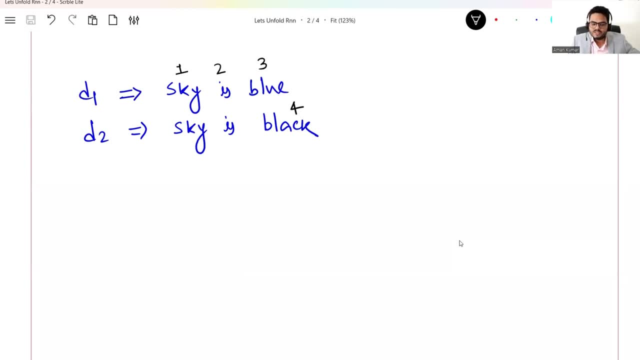 okay, now there is one very important concept that we have to understand when it comes to RNN, and the concept is known as time stamp, time stamp, okay. so one basic thing that will happen in RNN is: you don't send all these three words, for example, if I talk about the first record, or 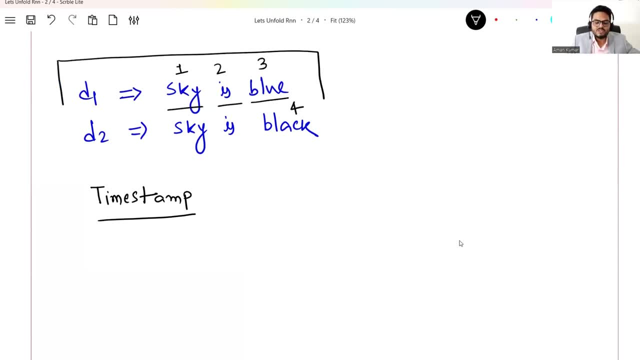 first document. so everybody, please pay attention here. the training will happen one document at a time, or one row at a time, right? so every time you talk of machine learning training, you talk of how this row will be trained, right? suppose this is a sentiment classification use case, right? so this is your, let's say, for example, target variable. this: 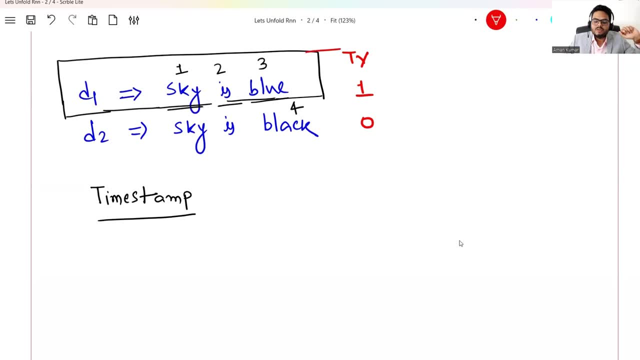 is, let's say, one, and this is, let's say, zero. so how the training will happen, this entire thing will be treated as one record, right? so when this first record goes in the network- try to understand this very carefully, guys, because this is base of R and N- okay, when the first record goes into the network, all these 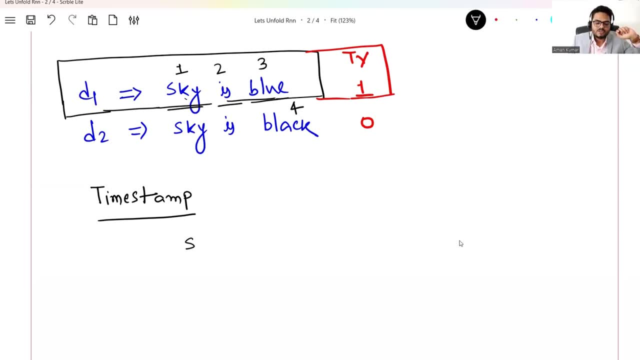 three words will not go together, okay, so first sky will go, first sky will go. let's call this time t minus 1. okay, then is will go. let's call this time t, and then blue will go. let's call this time t plus 1. so as you can see, here, in the same network, in the same input, in the 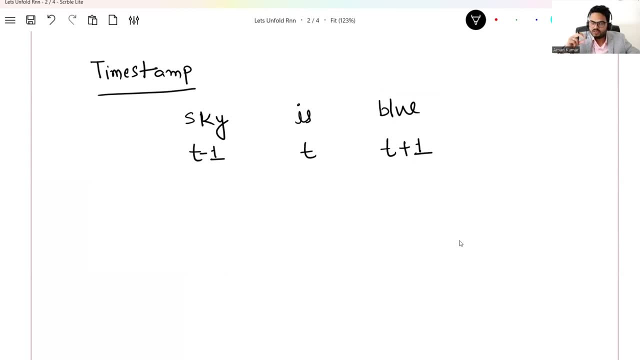 same you can say training of one single record, training. we are sending three words at three different time intervals. okay, three different times, and this concept in the world of R and N is called time stump. so at time stump, t minus 1, what is the input to the? 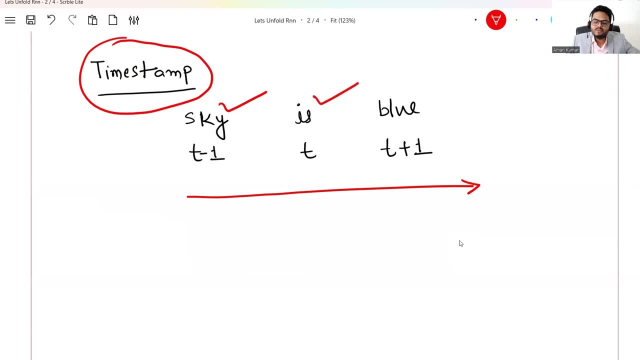 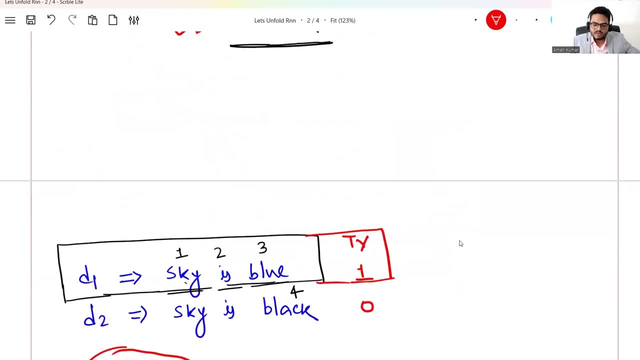 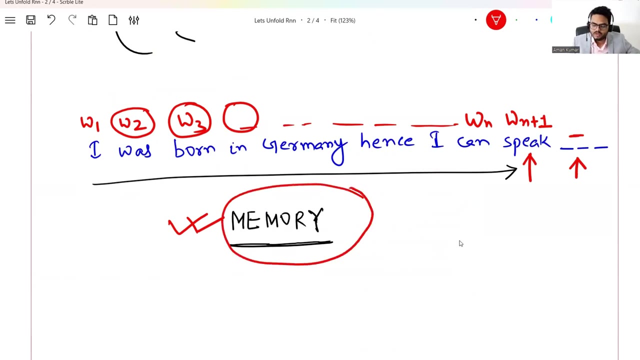 network sky. at time t: what is the input? is at time t plus 1. what is the input? blue. why this is important is every time we say that R and N remembers. so what is the one word that differentiates R and N from other networks? R and N has a memory, okay. so when we say memory that 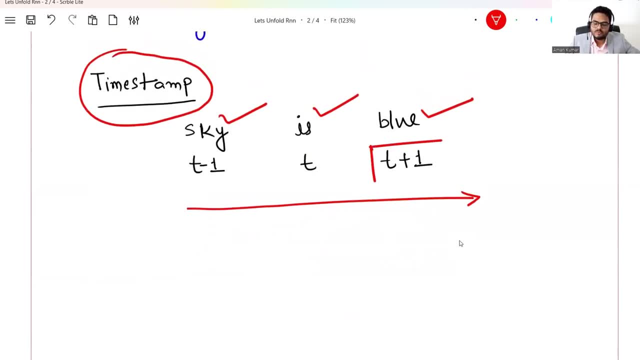 means that at time t plus 2, two things has already happened. what are those two things? one is sky and one is is. so R and N has a memory, okay? so when we say memory, that means that at time t plus 2, two things has already happened. so R and N will remember what happened at time t and what happened at time t. 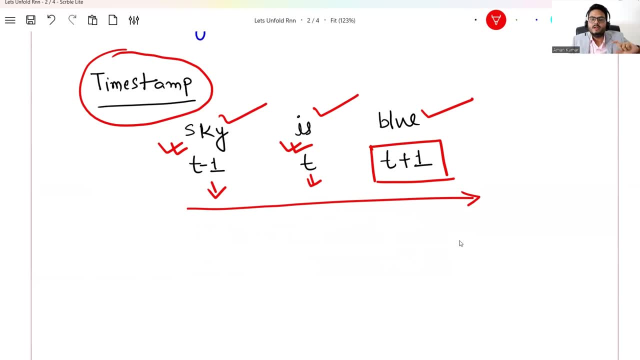 minus 1. that is what is called as the concept of time stump R and N. so I will come back to this. understand: time stump means when you send one word, that is your one time stump, and when you send the next word, that becomes time stump t plus 1. okay, just keep that in mind. we will come back. 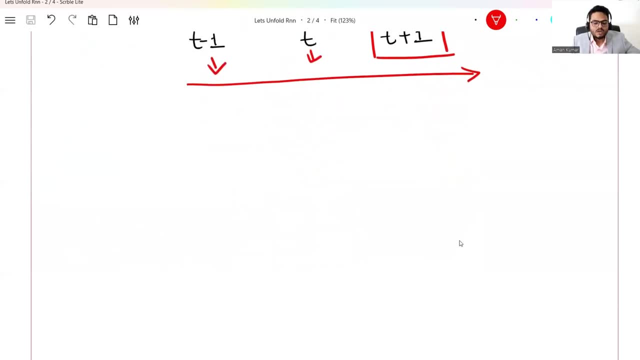 to this important concept, and now I will make it very, very clear to you how the pictorial representation of R and N changed. neural network changed when it came to R and N. so this is how typically a neural network looks. okay. so suppose I'll have four inputs. 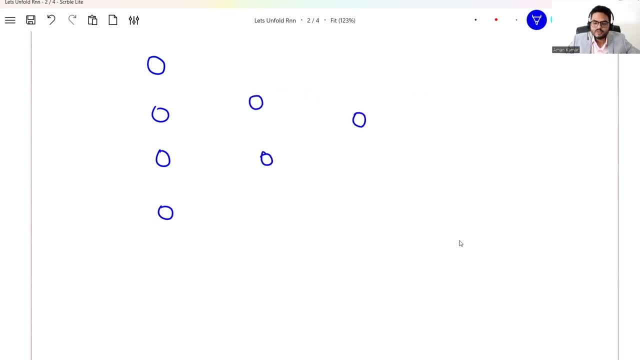 two hidden and one output nodes. okay, and I will just connect everything to everything. I will just connect everything to everything, because this is a fully connected neural network, so let me connect it. this is your neural network, okay? okay, so suppose this is a normal artificial neural network, not? 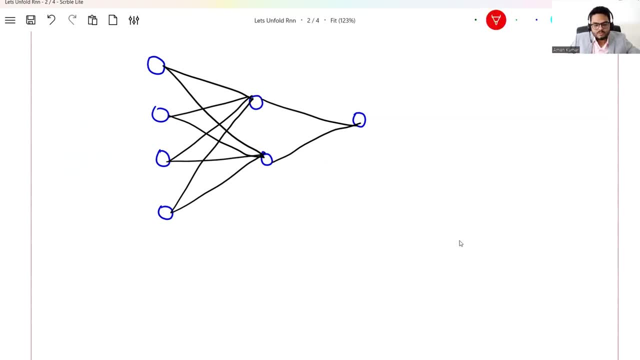 R and N. so what will happen? you just give your inputs from here, okay, and you take your outputs from here. this is your normal, simple, artificial neural network right now. just, you have to remember two things guys: what if? what? if I step one, I will do a two-step process here. step one is rotate, rotate anti-clockwise above picture. 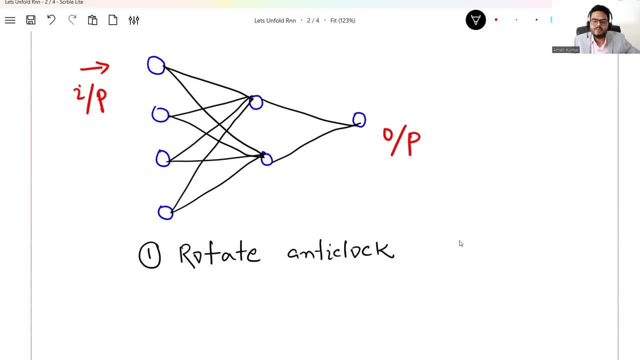 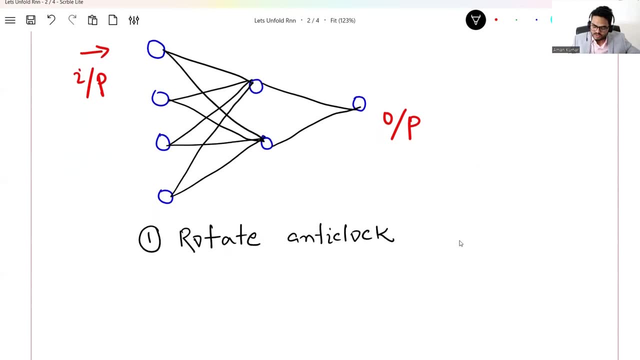 you rotate anti-clockwise. you can imagine if you rotate it anti-clockwise, then how it will rotate, not clockwise, anti-clockwise, like this. so if you rotate it anti-clockwise, then how your network will look. let me roughly draw it here: one, two, three, four, one, two and this is your output. 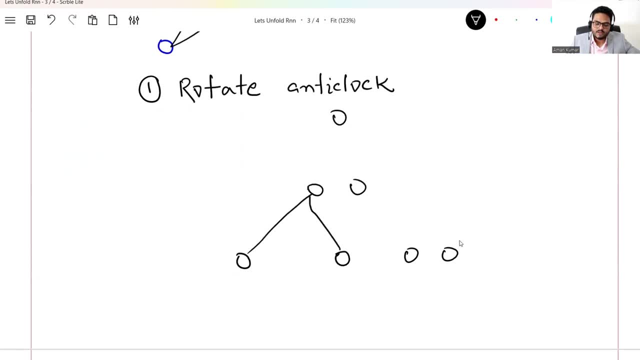 okay, so let me make it like this, so that you will be very clear on how the architecture of the R and N is looking like this. okay, so what? what I did now? I rotated anti-clockwise. okay, and then the second step you have to do is you have to shrink. the second step you have to do is: 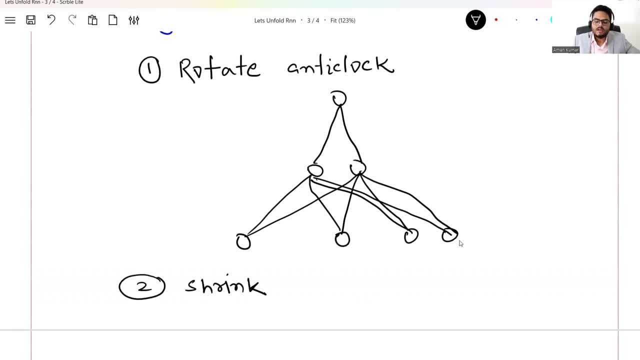 shrink s, h, r, i and k. now, at the moment, I shrink this, I squeeze this, right. so what you will see is this all thing I will squeeze and I will call this as input. okay, this I will squeeze and I will put this, put this inside a box and this, I will call that as an output, and 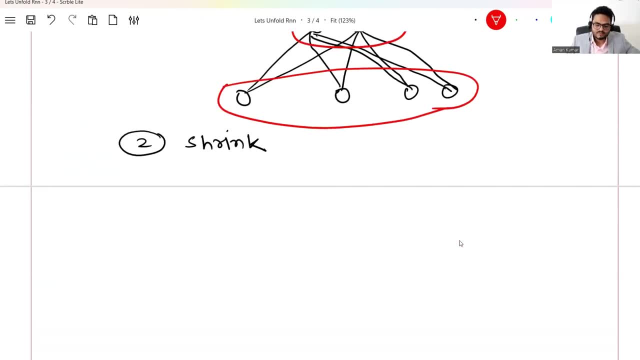 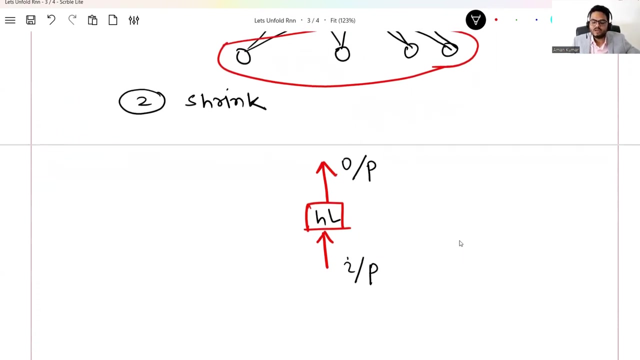 how I will represent this is like this: this is my input, okay, this is my hidden layer, okay, and this is my output. very simple to understand. nothing fancy here. so input: this is your output and this is your hidden layer, okay. so every time you see this picture and if you are confused that 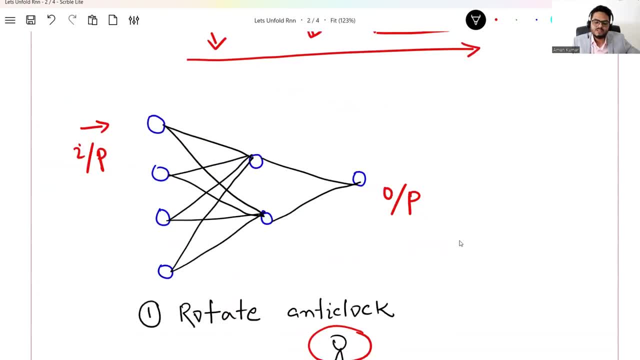 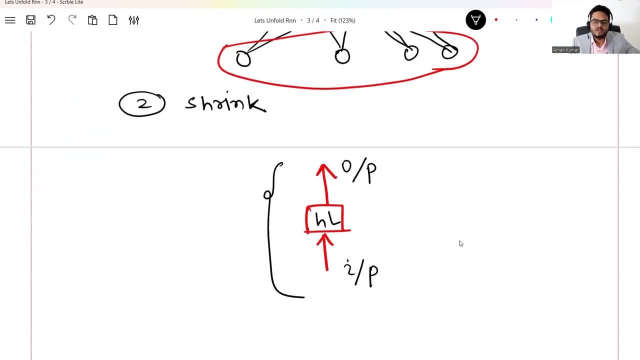 how neural network became like this. remember, this is the same neural network. we have just rotated anti-clockwise and we have squeezed it, okay, till now. this is not even R and N. this is simple, normal neural network, okay, so you have just rotated and squeezed it fine, up to here now, if you remember. 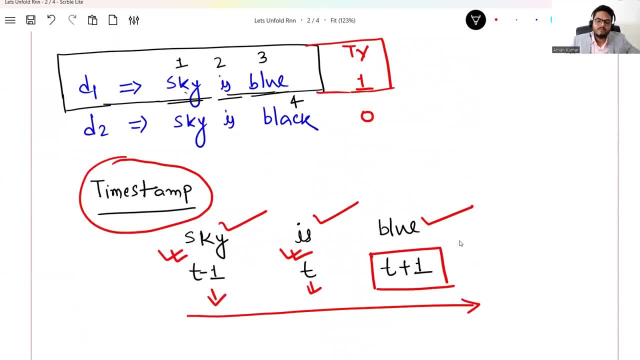 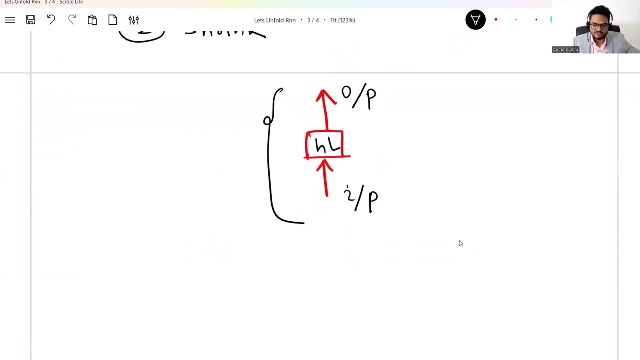 guys, I am telling you that R and N remembers the information of the previous state. so how that happens, let me explain you with a simple example. okay, so I will take the same neural network here, for example, this, this, this and this, and two nodes, okay, and I will just connect it again fully. 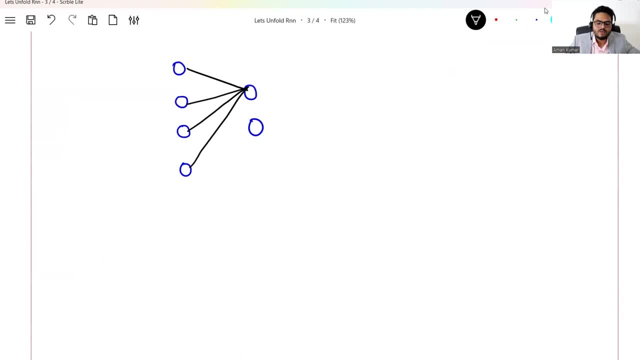 if I don't draw this again and again, then it will not be easy for you to understand. hence I am drawing it again and again. okay, so I am building the same network: four input, two hidden, one output. fine, suppose, suppose what is my first sentence? my first sentence is sky. sky is blue. right in my last video I told you 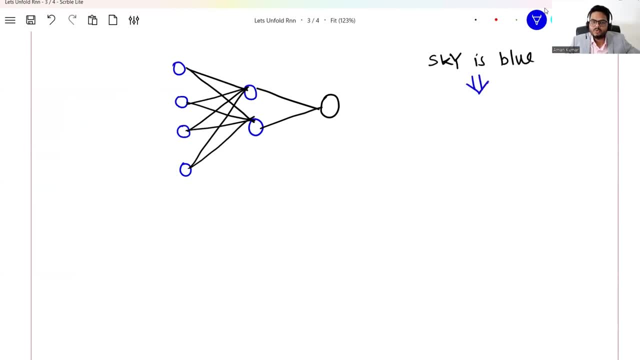 before training the model, we will convert it to some kind of encoding right. so suppose my vocab size is four and then I am drawing it again and again. okay, so I am building the same network four and sky is my first word. so one hot encoded vector of sky will be what? 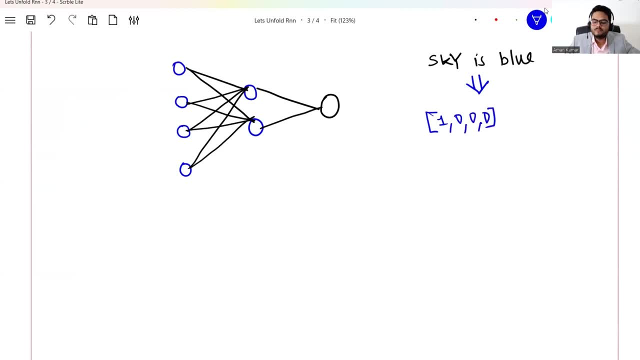 one, zero, zero, zero. right, one heart encoded vector of is will be what? zero one, zero, zero. now, somebody who is not understanding this, please? what the last video on, when I said NLP up to RNN? okay, so sky is being represented by this vector, one is being is being represented by this vector and blue. 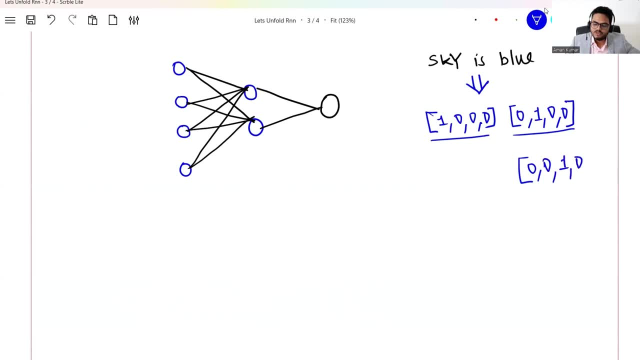 represented by 0, 0, 1, 0. okay, so my sentence- sky is blue- is now represented like this. fine, up to here. as i told you in rnn, input will go one by one. okay, so which word will go first? now suppose the first word that i send here is sky, so what will go as the input? guys? 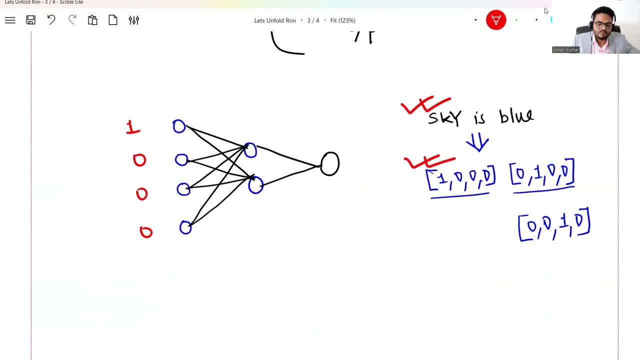 1 0 0, 0. this goes as the input, right, and then there will be weights. there will be weights, right. so how many weights will be here? how many weights will be here? you can comment me down how many weights will be here. i'm not writing how many weights will be here from input to hidden. 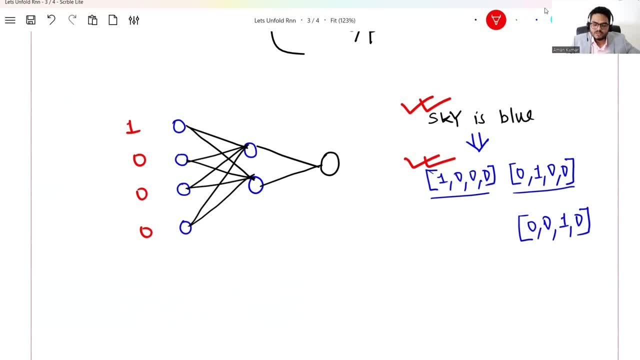 and suppose these weights goes here and then activation function works here okay on weights and biases and then some output comes. fine, what? Whatever the output comes right, that output will go here and the same output will come back to the node as well, and same output will go to the other node as well, hidden node similarly. 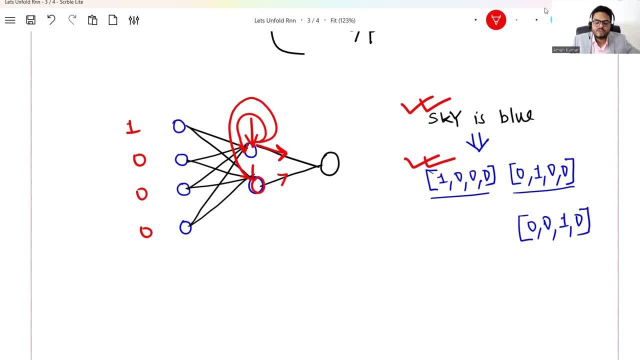 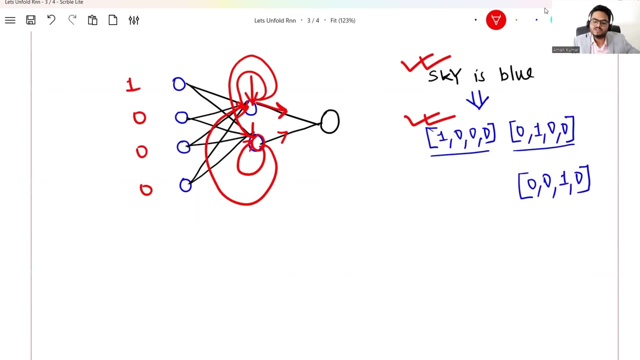 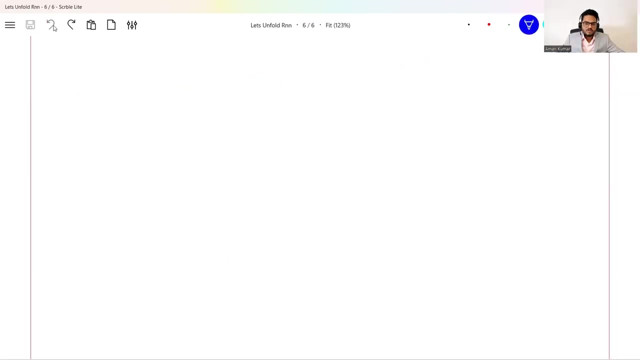 whatever output comes from this hidden node, this output comes back to this hidden node and this output goes back to another hidden node as well. okay, I know this diagram is becoming complex, and that is the reason. I will explain you in two levels how this is happening. okay, so let me omit this first. let me omit this first. 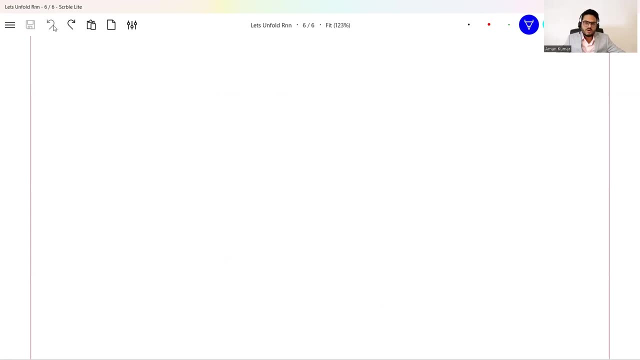 So if you have understood up to here, then it's a cakewalk to understand how RNN works. Let's write our three words here. so first word is Sky, second word is is and third word word is blue. okay, so, as i told you, all these world will go into the network one by one, so let's draw. 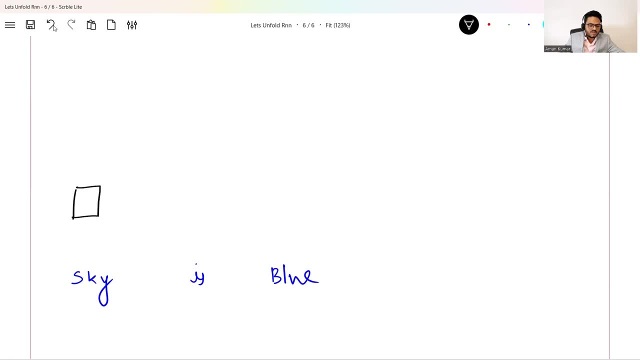 our network here. so this will be my network, the squeezed form of the network, not the expanded form. okay, then again, same network, but a copy of the network. when is word comes? same network, but at a different time state: okay. and same network, but at a increased time stamp or time state: okay. so for 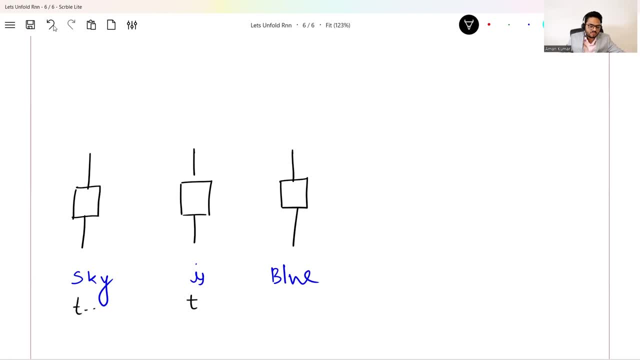 example, this can be my t, this can be my t minus 1 and this can be my t plus 1. so same network at three different time steps or time stamps. okay, so here when the sky word goes into the network, it will go with some weight right, and then activation function will work on this weight. 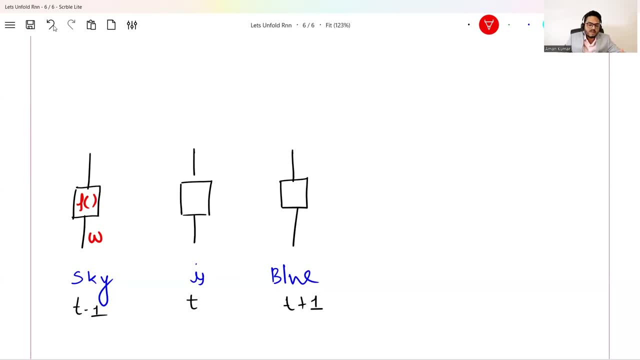 multiplied by sky's vector plus some bias, and you get some output right. the only difference between normal neural network and i, i, rnn is rnn will pass this output. let's call this o1 to the next state. next state means when the next word enters into the network. so o1 will come and again the vector of is will come and the 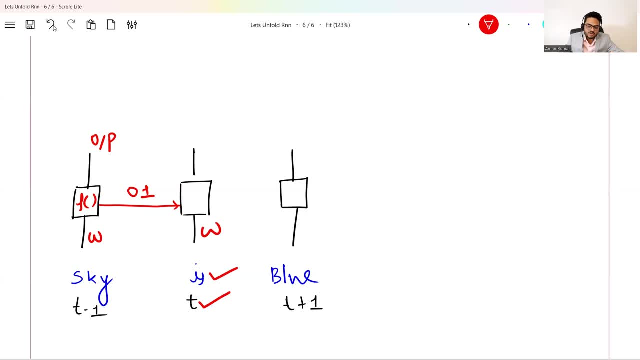 weight will come as usual. right, so this is one input. the w weight multiplied by is vector and other input. at this step, this is very important to understand. at this hidden layer, the function will become output. 1. multiplied by this, output will also come with some weight. okay, so let's call that weight 1. 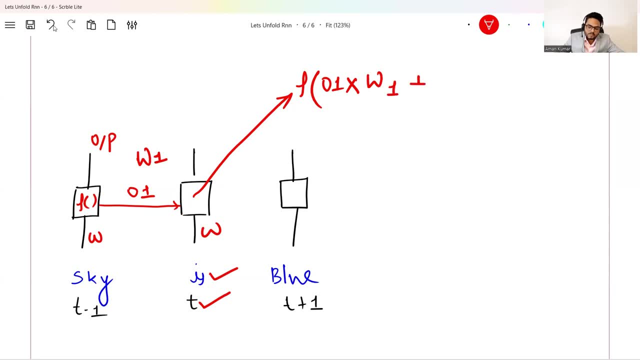 so output: 1 multiplied by weight, 1 plus. this is vector. so i will say vector of is multiplied by w plus bias. okay, this f is nothing but your activation function and let's say this output is o2. so next time, at next time, stamp what will happen in the network. again, this blue.